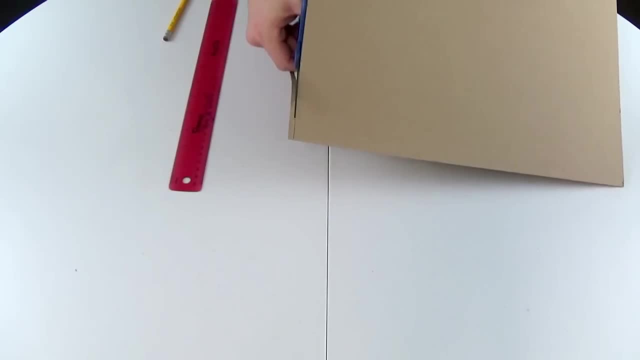 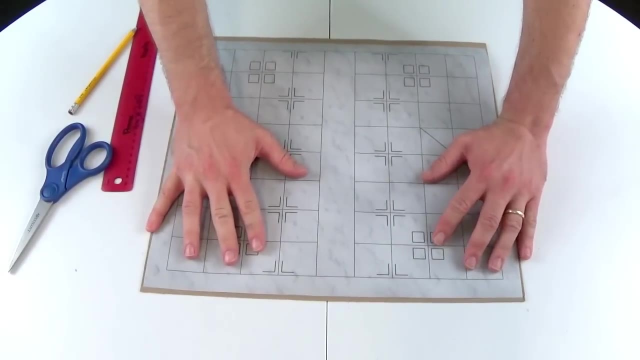 Measuring four layers with a ruler gives me an eighth of an inch, which is what I'll trim off the edge. As you can see, the far edges are now much closer to our printout's width. So we're committed to this course, which sucks if you struggle with commitment. Why do they? 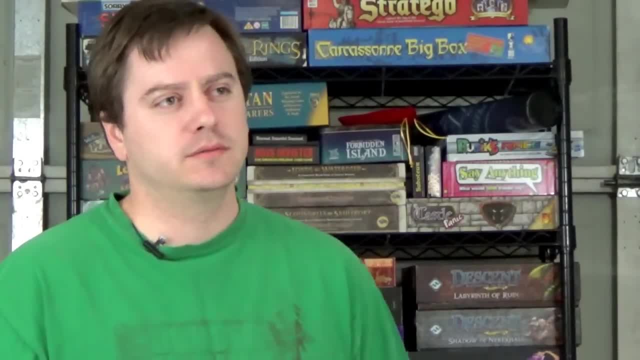 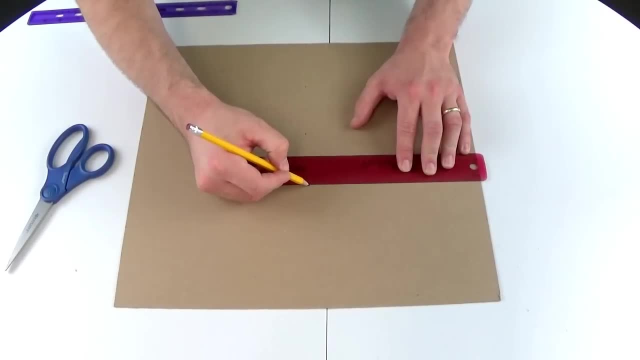 call it a bifolding board when it's only got one fold. Now take this backing and cut it exactly in half Measure from the bottom to the top and cut it exactly in half Measure from both sides. if you need to ensure an equidistant cut, Precision is important, which. 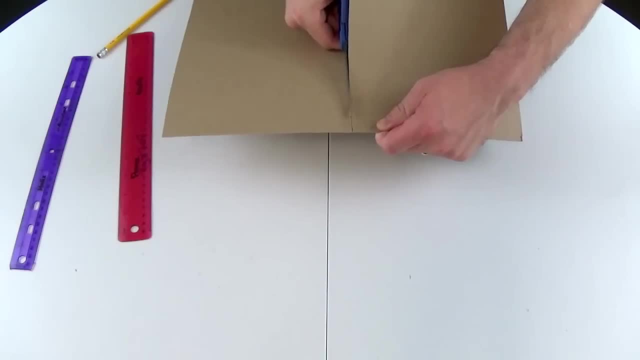 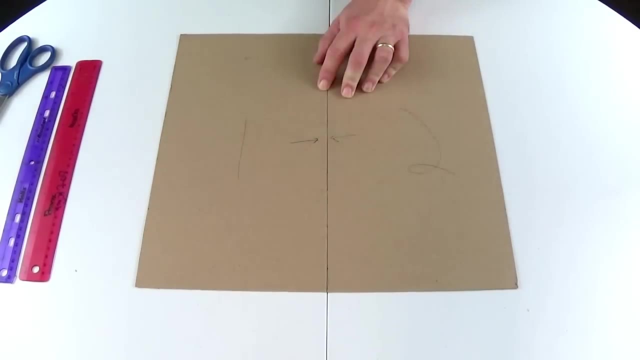 is why I score my line with the blunt edge of the scissors. before I make the cut, Now check your hemiplanes and mark the direction of their configurations. The next task is a bit redundant: Score and cut identical copies of the board's sides and identify these as 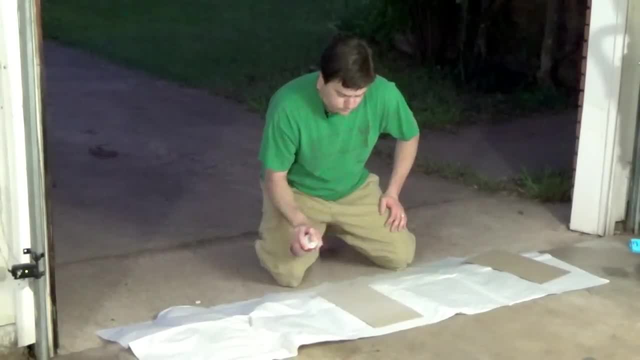 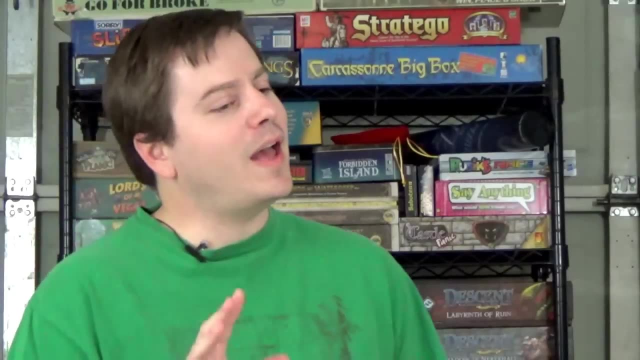 second layers. Then use the spray glue on one of each side's hemiplanes and glue the congruent sides together, doubling the layers. No, no, I know it has two sections, but the bi is prefixing the fold, not the sections. 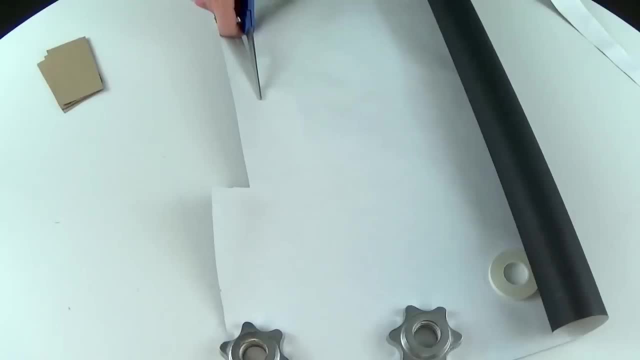 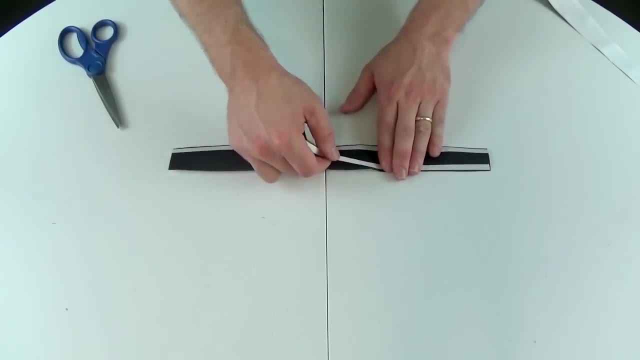 We don't call it a bi-sectional board. Cut a couple of one inch wide strips from the backing paper, Use the bookbinding tape and line the long edges of these strips. In my example, I'm lining one strip on the dark side and the other one on the white side due. 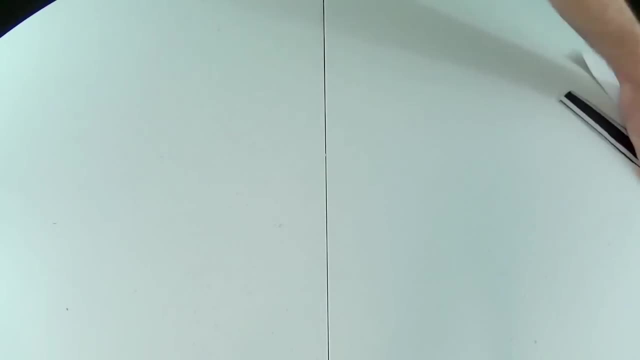 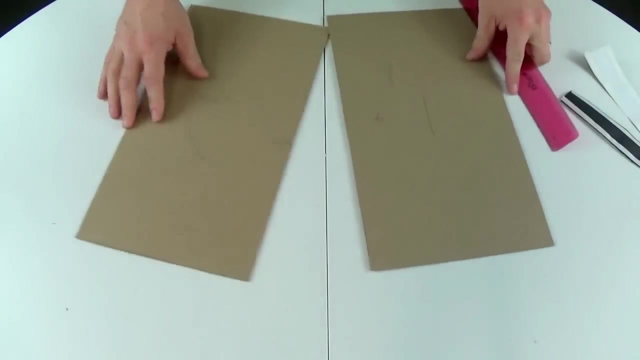 to the dark and light colors used on the front and back sides of my final board. So what would we call the non-folding board? Like a monoboard? Remember when we trimmed our edge down? Well, here is where we make that space back, Separate the two sides slightly. 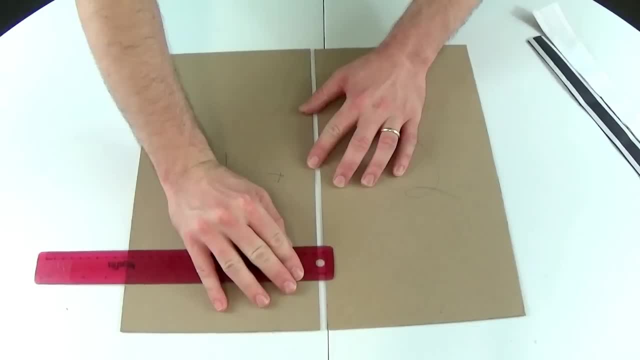 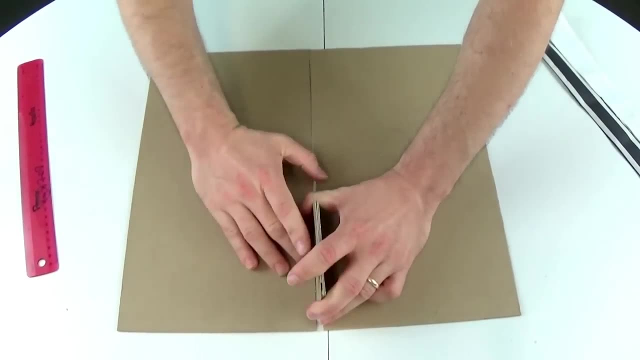 more than the total thickness of all four layers pressed together. Now, keeping these apart is tough, so I brought in five of those chipboard scraps to act as spaces to hold my place. Yeah, longer spacers would have been better, but I use these super small ones. 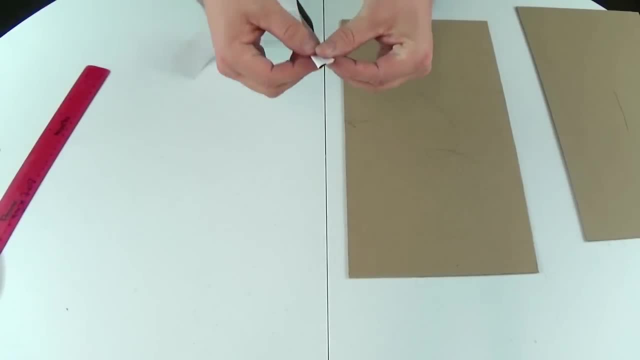 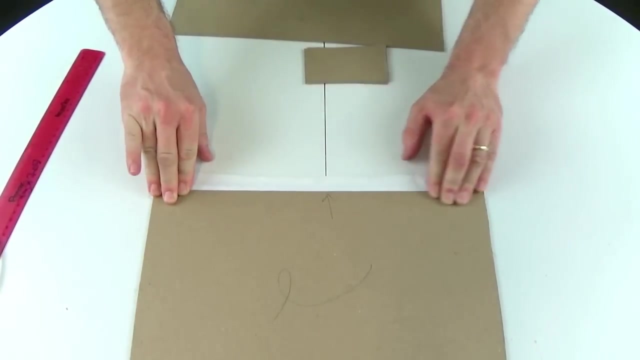 anyway, stop judging me. Fold the back sides matching strip in half, Hot dog style. That's long ways for you amateurs. Peel off the wax on one side's score tape and use a couple of those chipboard placeholders to space the chipboard halfway from the strip's centerfold, Pressing a hemi-plane evenly along. 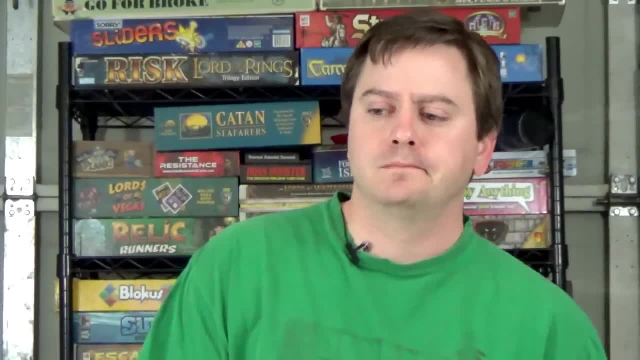 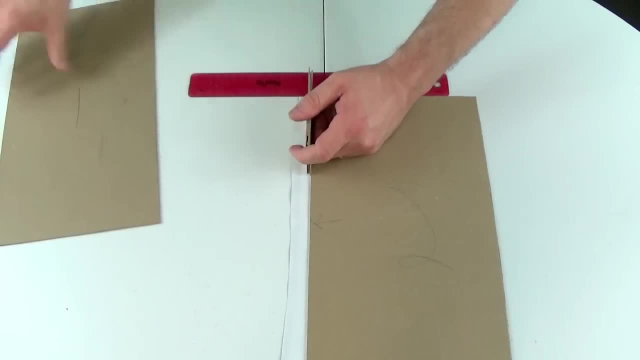 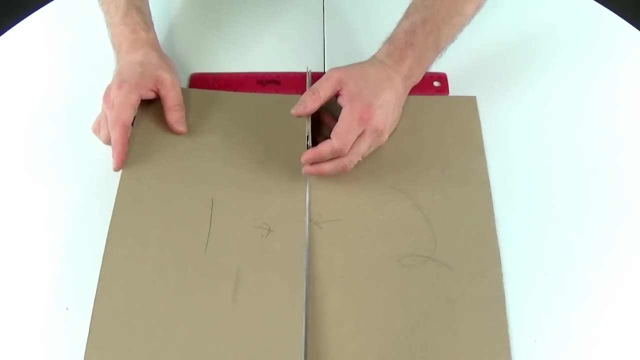 the strip Null fold. What about Latin? Ah, folding board. Now, with the other side's wax tape removed, use all the appropriate spacers to space out the other half of the board from the other half of the board. Hey, that's great writing there, riders. 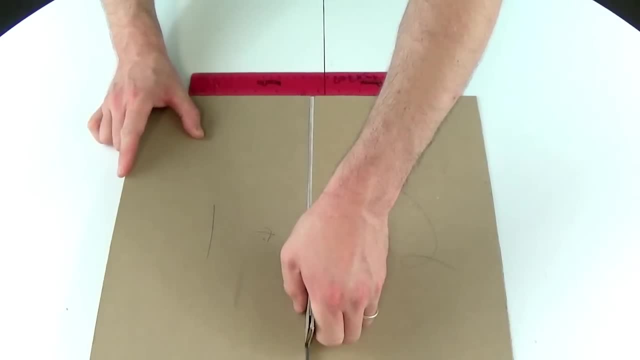 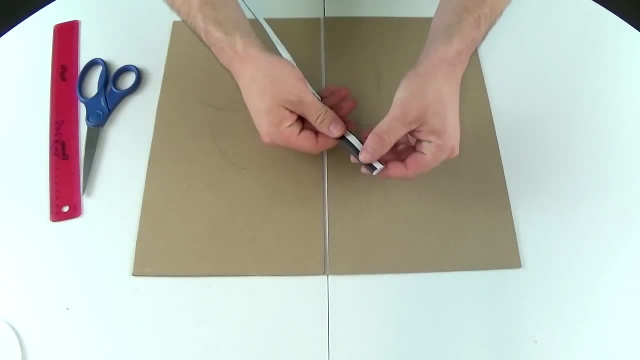 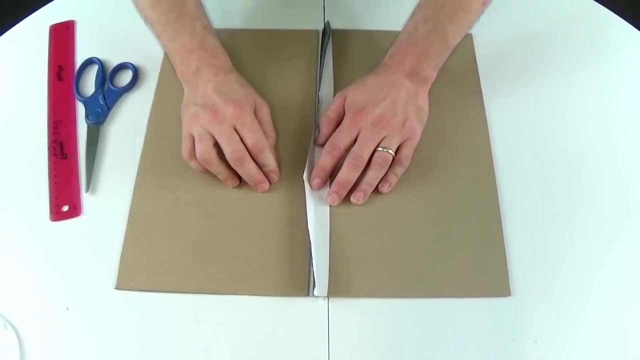 Use a straight edge along the top edge to keep the board edges aligned and even. And the great writing continues. Trim your strips and prepare the second strip for the front side. This time, use the fold as a guide to keep the strip centered, letting the fold of the strip tuck into the trench. 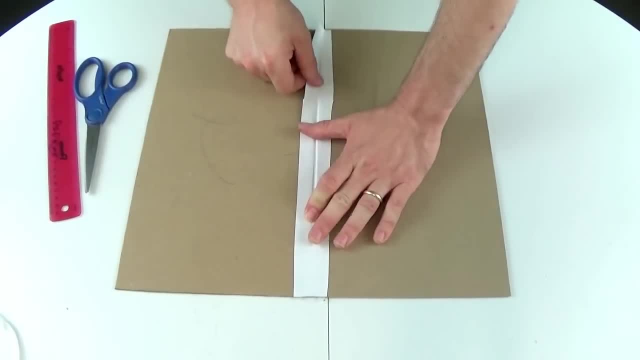 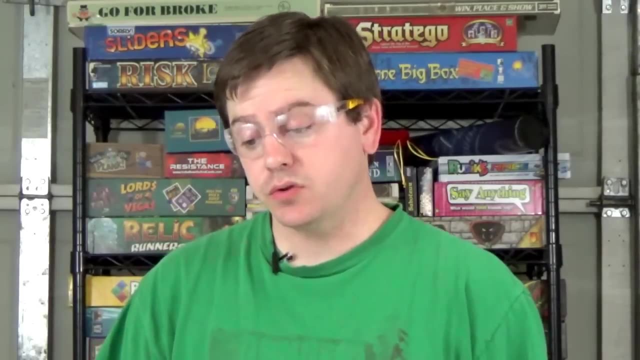 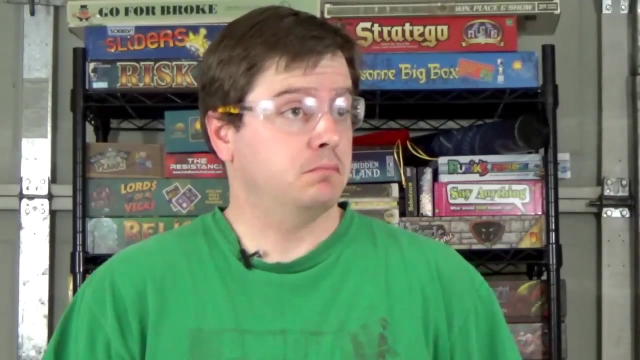 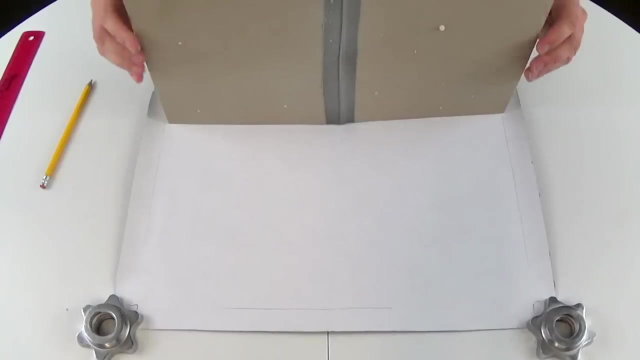 a bit before full adhesive-sy acquired. Is that even a word? When closed, the board should match up perfectly. Bicycle is two sickles. unicycle cycle, uniboard, Uniboard. Okay, so wrap the backing paper as we did in our uniboard video by giving a one-inch frame to work. 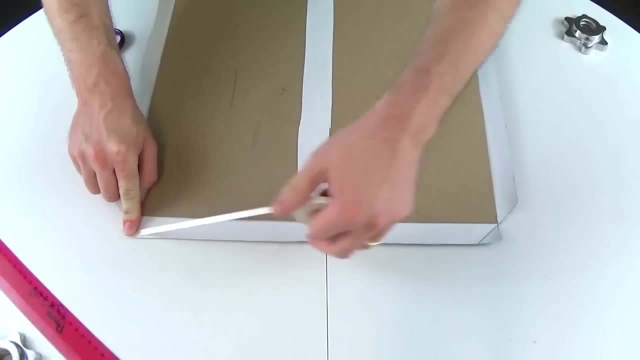 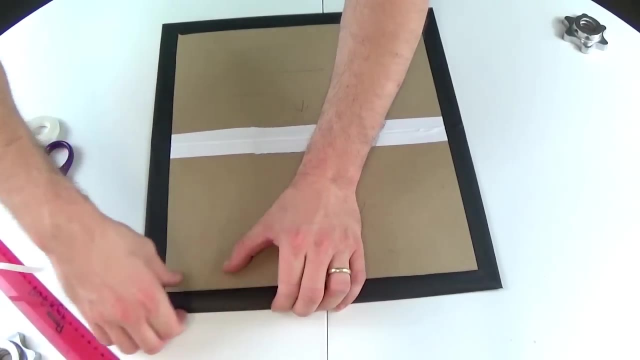 with Spray glue and mount the chipboard, finishing by wrapping the edges. For an in-depth detail on this process, go check out DIY's how to make a game board- the prequel, starring yours truly, If your board halves are thicker than the one I'm. 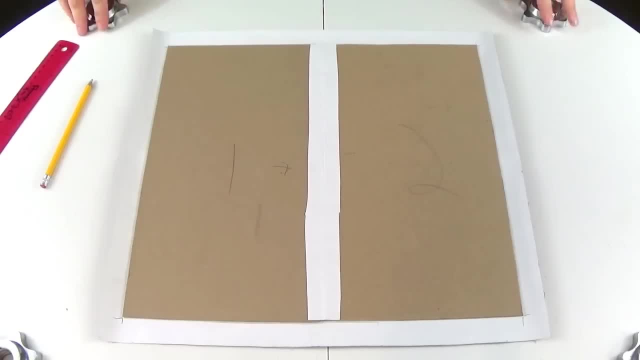 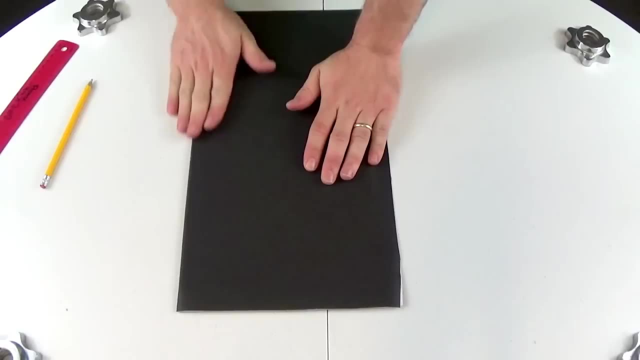 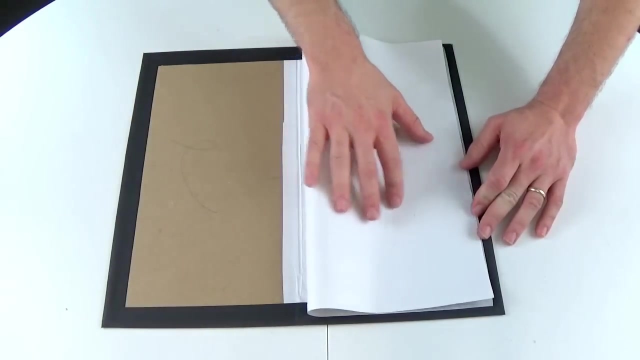 making here or your backing material isn't as forgiving, you'll want to wrap your backing around the hinge as well, rather than pressing this flat. or, even better, look to our tri-fold method, which allows for a separation in the backing material. Now, once wrapped, take your print out and fold it in half to match. 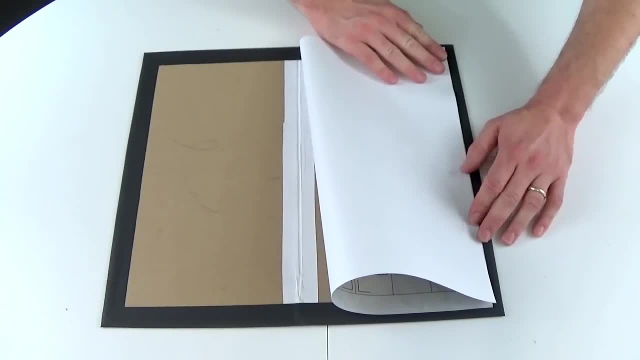 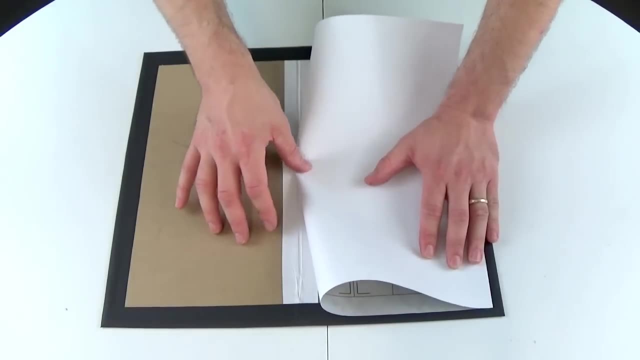 the trench. run in our bi-folding board and don't be cavalier about this fold. okay, it's the fold that tells everyone playing your game: hey, this guy or girl is both attractive and well adjusted. so enjoy yourselves and play this game. Use the glue stick on the. 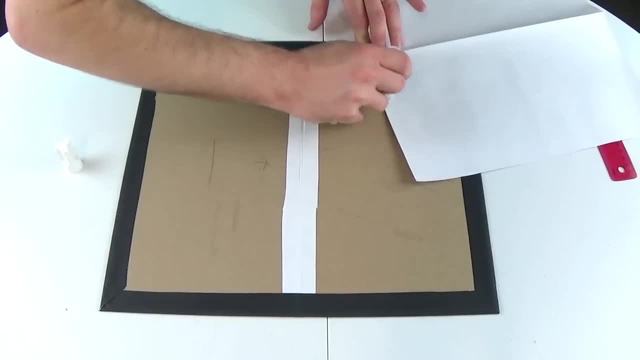 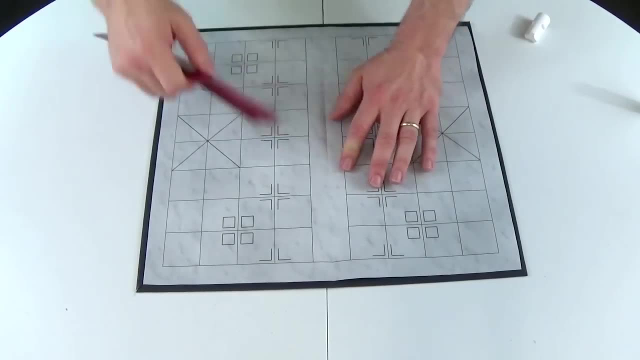 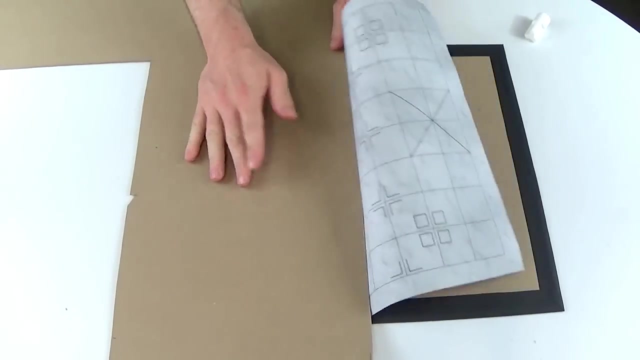 backside of one half of the printout, making sure you nail these edges in the center fold with the glue stick. Now line this up as perfectly as superhumanly possible and attach the board adhering from the center out. Now repeat this for the other half, using some scrap material to back up the edges, for.